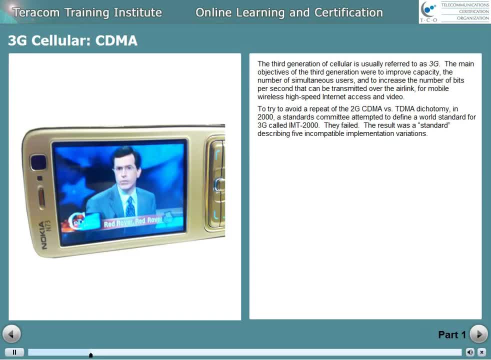 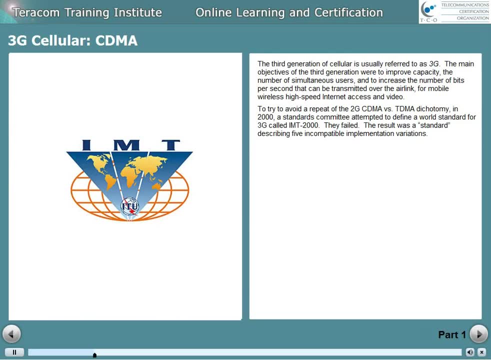 To try to avoid a 3G data communication technology. we're going to talk about the 3G data communication technology. More information on that coming up in the second part of today's presentation. Results of understanding of the 2G CDMA versus TDMA dichotomy In 2000: a Standards Committee. 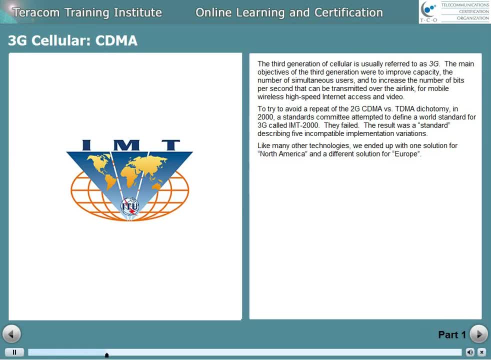 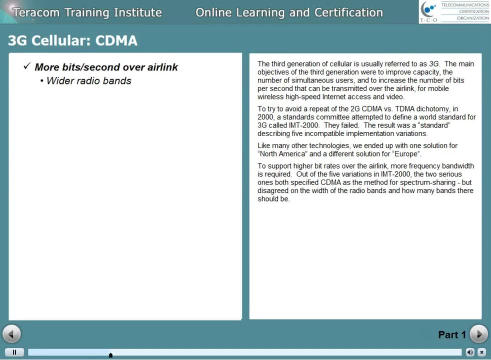 attempted with one solution for North America and a different solution for the rest of the world which is called Europe. in the telecom business, To support higher bit rates over the air link, more frequency bandwidth is required Out of the five variations in IMT 2000,. 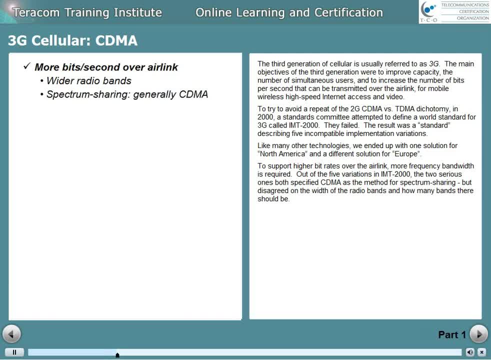 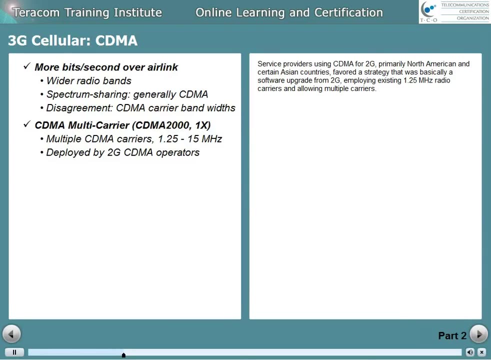 the two serious ones. both specified CDMA as the method for spectrum sharing, but they disagreed on the width of the radio bands and how many bands there should be Service providers using CDMA for 2G, that's primarily North American and a few Asian countries. 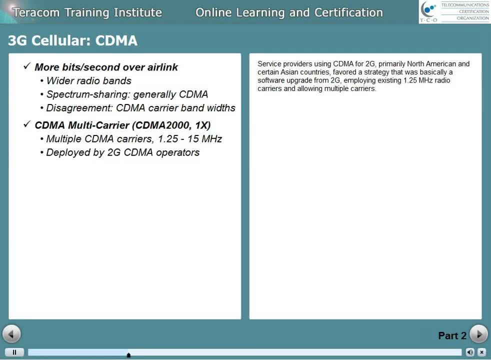 favored a strategy that was basically a software upgrade from 2G, employing the existing 1.25 MHz radio carriers and allowing multiple carriers. This is called IMT-MC multi-carrier CDMA- Qualcomm's brand name, and the name for this was CDMA-2000.. 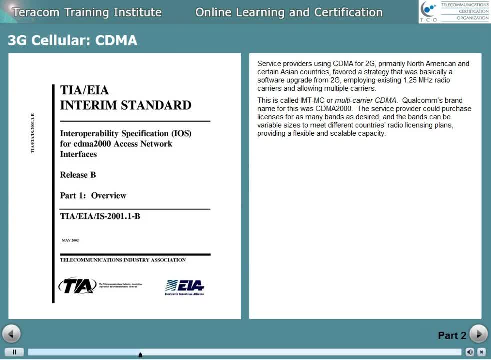 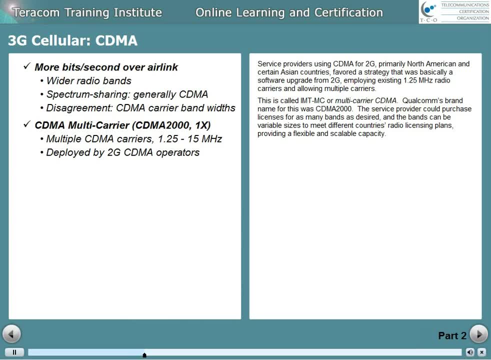 This was Qualcomm technology, basically an upgrade from 2G to 3G, And in fact, their 2G chips already implemented this, so it wasn't a big leap. The service provider could purchase licenses for as many bands as desired. 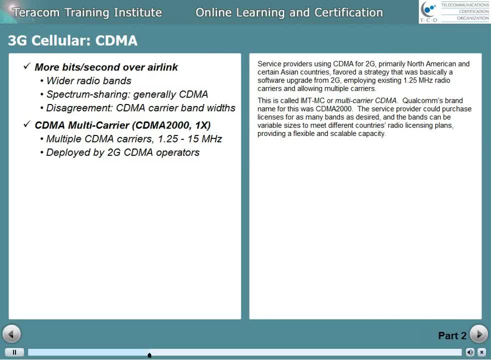 and the bands could be variable sizes to meet different countries' radio licensing plans, and it provided a flexible and scalable capacity. A single 1.25 MHz carrier- a carrier version of this referred to as 1X- was widely deployed- Now service providers using GSM-TDMA for second generation. 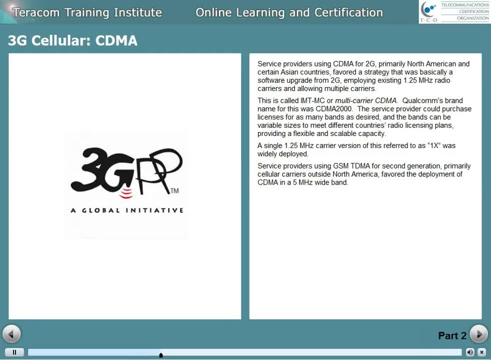 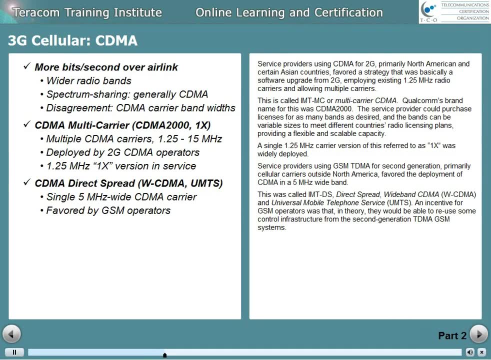 which is primarily cellular carriers outside North America, favored the deployment of CDMA in a 5 MHz wideband. This was called IMT-DS direct spread. It was also called wideband CDMA and universal mobile telephone service, UMTS. 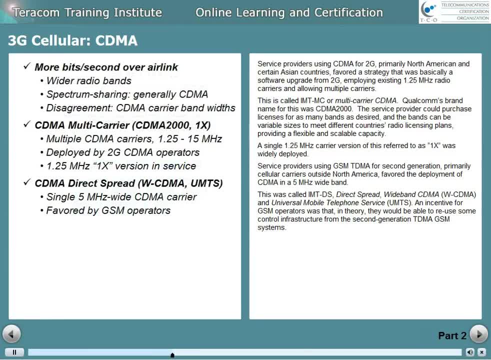 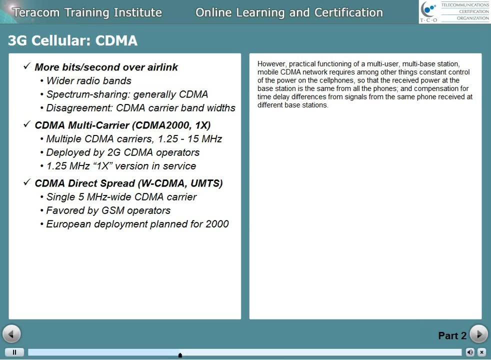 An incentive for GSM operators was that they, in theory, would be able to reuse some control infrastructure from second generation GSM systems. However, practical functioning of a multi-user, multi-base station mobile CDMA network requires, among other things, constant control of the power on the cell phones. 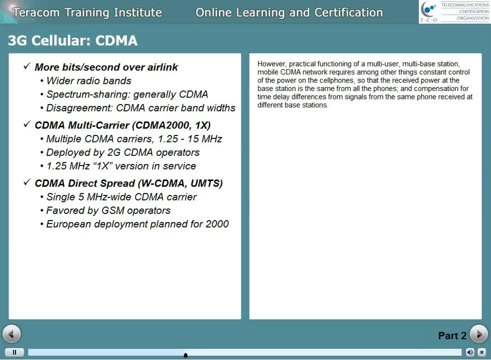 so that the received power at the base station is the same from all the phones, regardless of how far away they are. the received power is the same. This means you have to turn the power up and down on the phones And we also have to compensate for time delay differences. 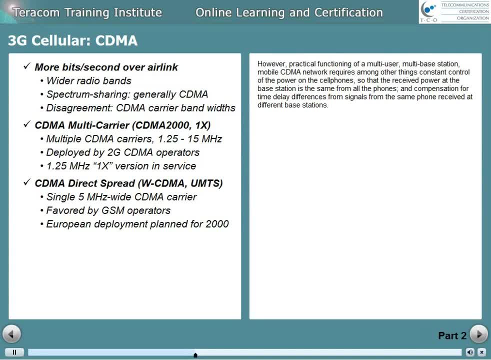 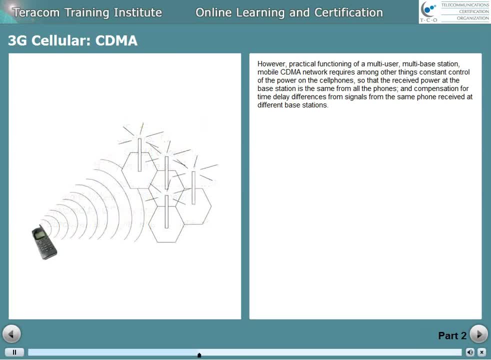 from signals from the same phone received at different base stations. CDMA is mind-boggling stuff and when you're doing CDMA you're not just talking to one base station, you're talking to all of them, and all of them report their answers. 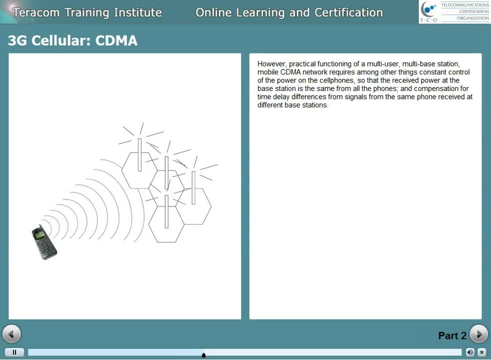 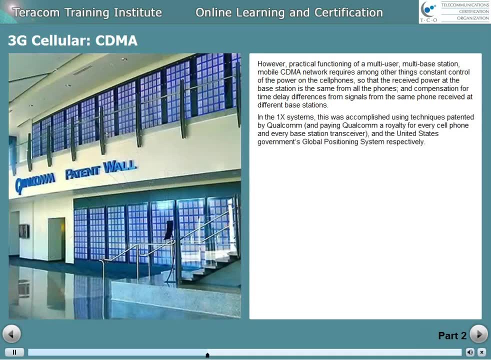 All of the answers back to the mobile switch and it has to weight them and to do that it has to correct for time delay differences In the 1X systems. this was accomplished using techniques patented by Qualcomm and paying Qualcomm a royalty. 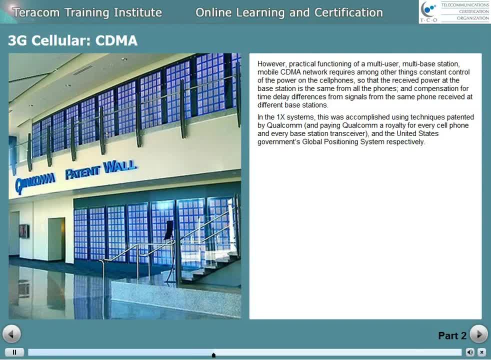 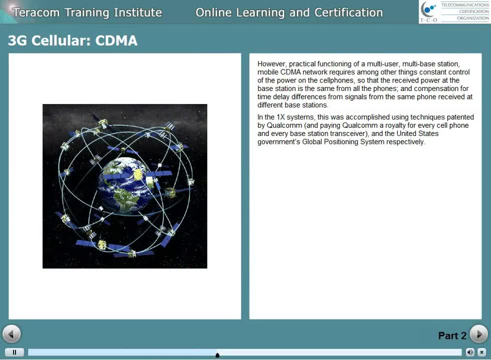 for every cell phone and every base station transceiver and using the United States government's Global Positioning System. Every CDMA cell phone has a GPS chip in it so that the switch knows where the phone is and can calculate the distance between the phone. 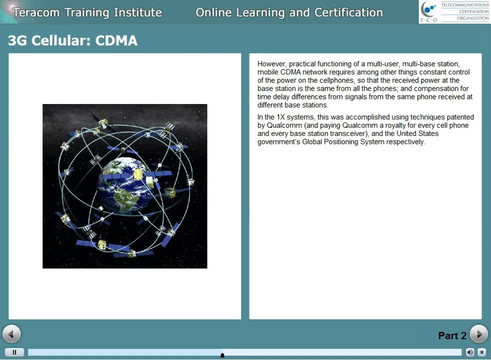 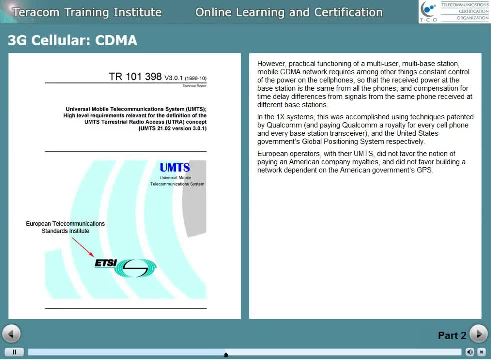 and every one of the base stations to correct for time delay differences. Now, European operators, with their UMTS, did not favor the notion of paying an American company royalties and did not favor building a network dependent on the American government's GPS. Also, since UMTS required mathematical calculations, 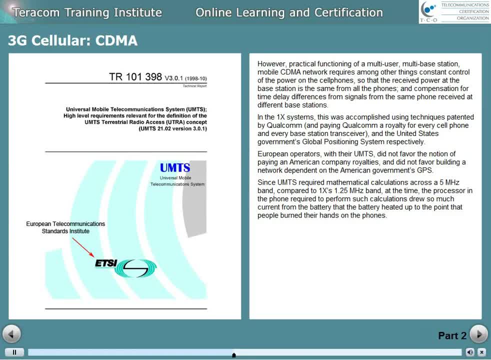 across a 5 MHz band, compared to 1X's 1.25 MHz band. at the time, the processor in the phone required to perform such calculations drew so much current out of the battery that the batteries in the phone heated up. 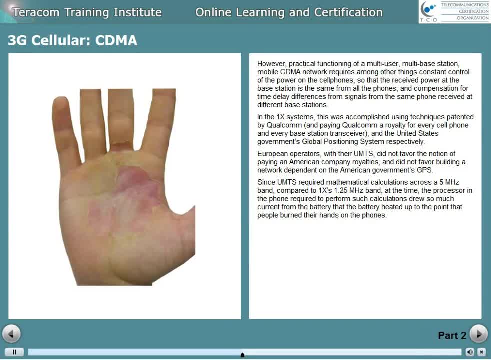 to the point that people burned their hands on the phones during trials, and I'm not making this up. The GSM UMTS Europeans then embarked on a seven-year-long odyssey attempting to circumvent Qualcomm patents and avoid using GPS. After a number of strategies failed, 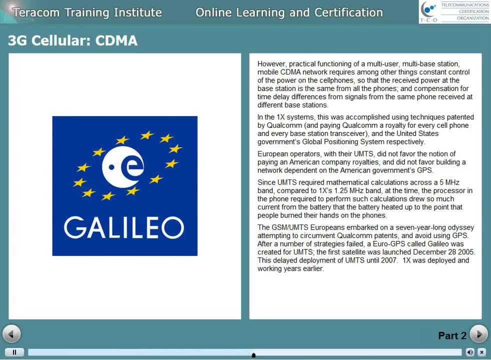 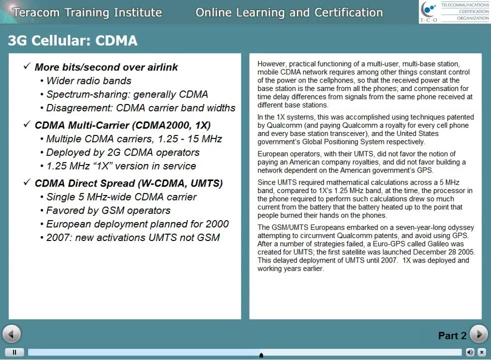 a Euro GPS called Galileo was created for UMTS. The first satellite was launched on December 28, 2005.. This delayed the deployment of UMTS until 2007.. 1X was deployed and working years earlier, The tipping point between 2G and 3G. 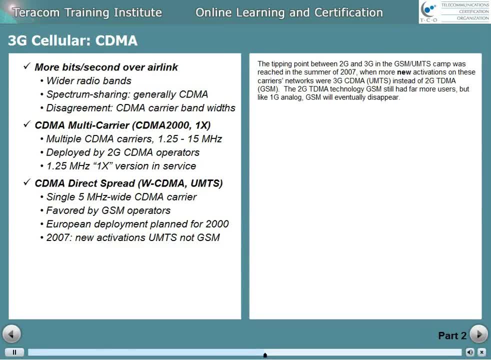 in the GSM UMTS world was reached in the summer of 2007.. When more new activations on these carriers' networks were 3G CDMA, that's UMTS, instead of the 2G TDMA, which was GSM. 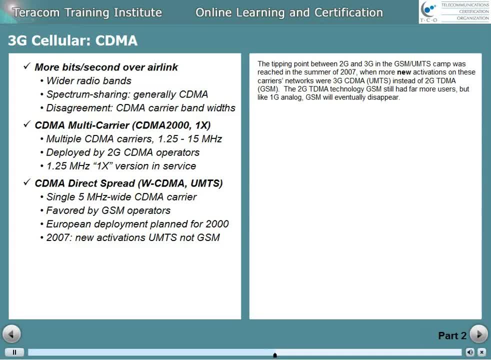 Now that doesn't mean that in 2007 there were more UMTS phones than GSM phones. No, no, It meant that new activations were 3G instead of 2G. The 2G technology- GSM- still had far more users. 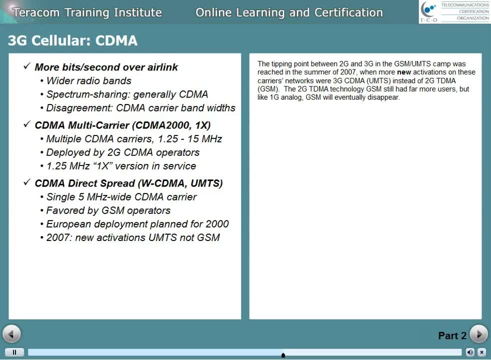 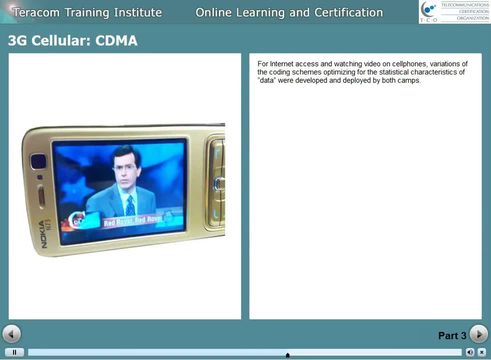 but, like 1G, analog GSM will eventually disappear For internet access and watching video on cell phones. variations of the coding schemes optimizing the statistical characteristics of data were developed and deployed by both camps. In both cases, these were deployed on carriers. 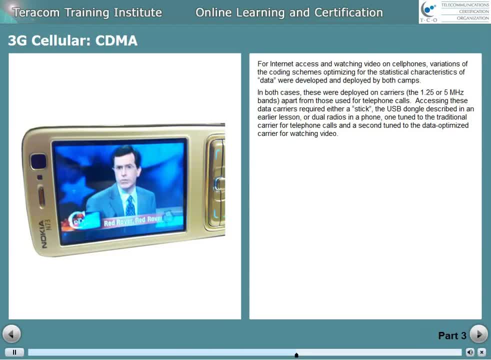 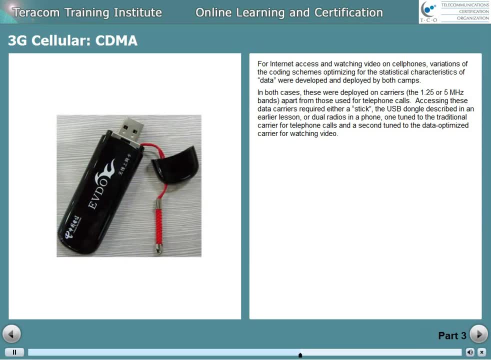 These are the 1.25 or 5 MHz wide bands that were different than the ones used for telephone calls. Accessing these data carriers required either a stick- the USB dongle described in an earlier lesson- or dual radios in a phone. 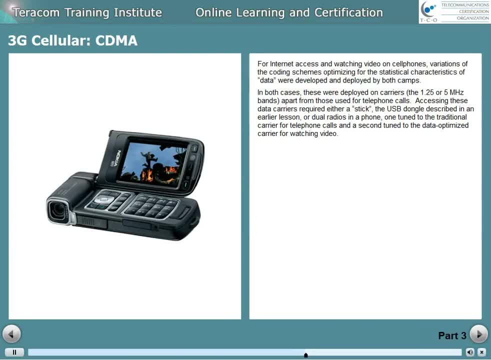 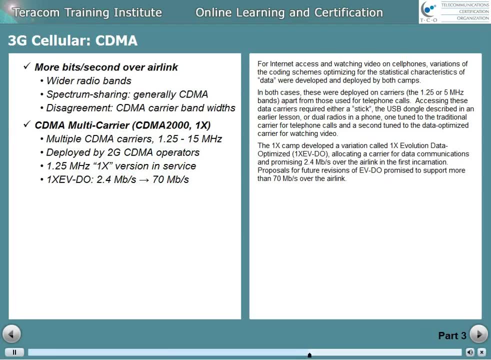 one tuned to the traditional carrier for voice and the other one tuned to the data carrier for watching video. The 1X camp developed a variation called 1X, Evolution, Data Optimized, 1X, EVDO And, by the way, it's called 1X. 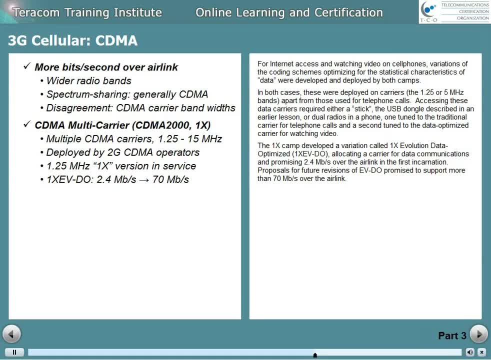 because they used one 1.25 MHz wide carrier, The 1X. EVDO allocated a carrier for data communications and at the beginning they promised 2.4 Mbps over the air link. Proposals for future revisions of EVDO promised to support more than 70 Mbps. 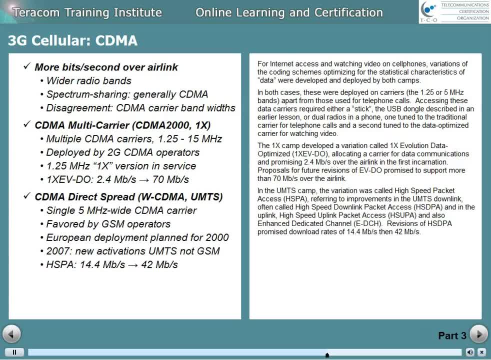 over the air link. In the UMTS camp the variation was called High Speed Packet Access And that referred to improvements in the UMTS downlink, often called High Speed Downlink Packet Access, and in the uplink the High Speed Uplink Packet Access. 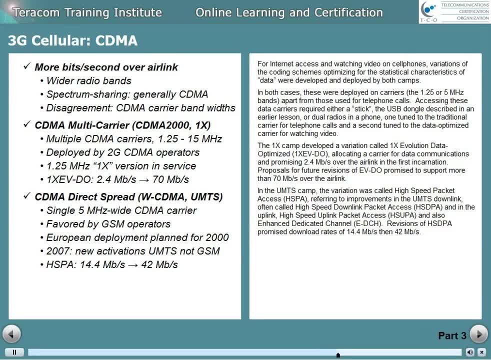 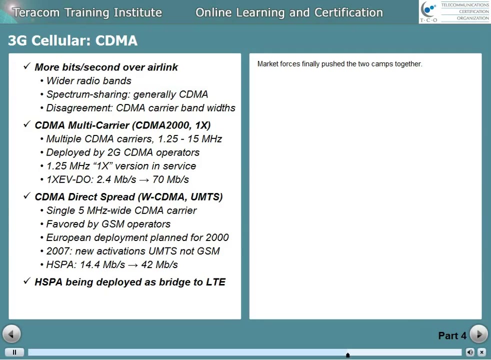 and also enhanced dedicated channel Revisions of HSDPA promised download rates of 14.4 Mbps, then 42 Mbps. later on, Market forces finally pushed the two camps together: The fact that there were far more 2G GSM users on the planet. 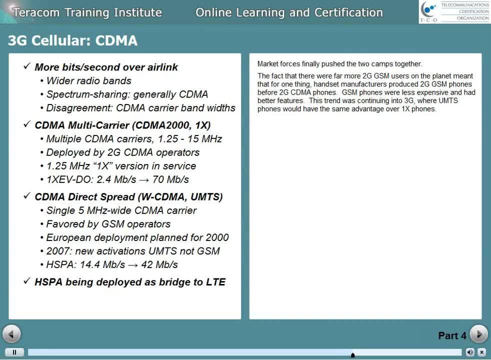 meant that, for one thing, handset manufacturers produced second generation GSM phones before second generation CDMA phones. GSM phones were less expensive and they had better features. This trend was continuing in the third generation, where UMTS phones would have the same advantage over 1X phones. 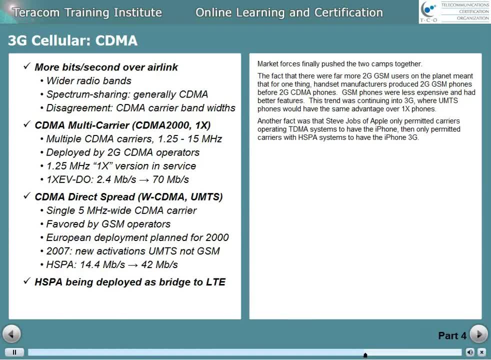 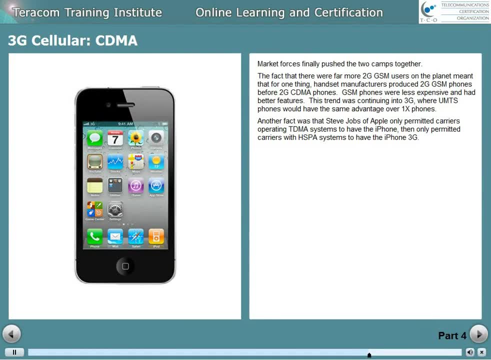 Another fact was that Steve Jobs of Apple only permitted carriers operating TDMA systems to have the iPhone, then only permitted carriers with HSPA systems to have the iPhone 3G. Finally, the 1X camp threw in the towel and decided to go with. 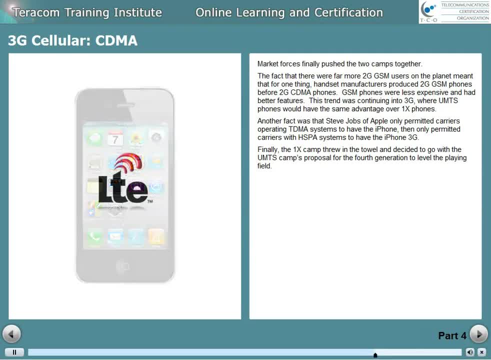 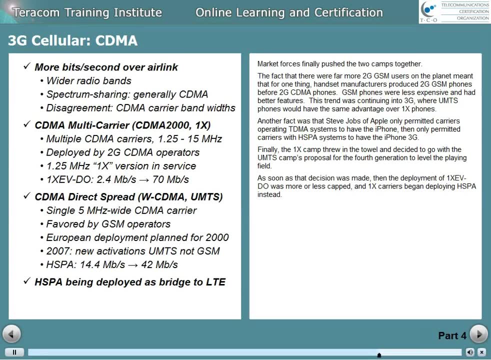 the UMTS camp's proposal for the fourth generation to level the playing field. As soon as that decision was made, the deployment of 1X EVDO was more or less capped and 1X carriers began deploying HSPA instead of the 1X EVDO. 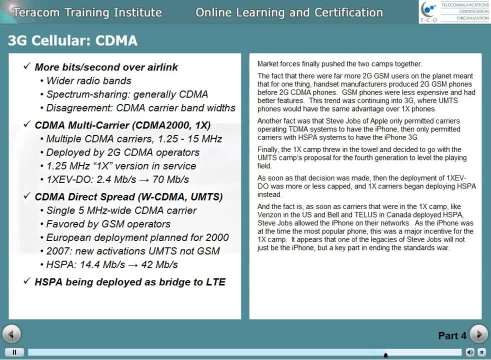 And the fact is, as soon as carriers that were in the 1X camp, like Verizon in the US and Bell and Telus in Canada, deployed HSPA, Steve Jobs allowed the iPhone on their networks, As the iPhone was, at the time, the most popular phone. 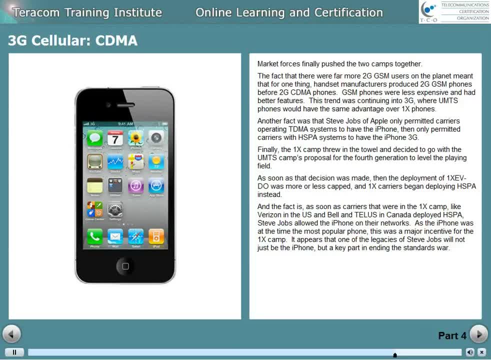 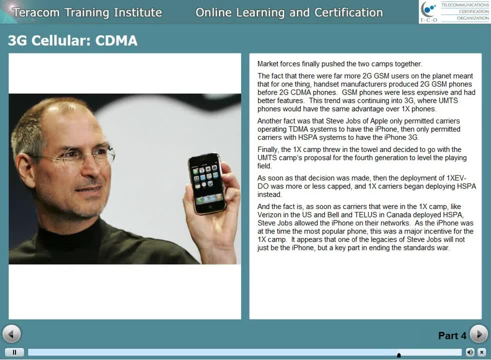 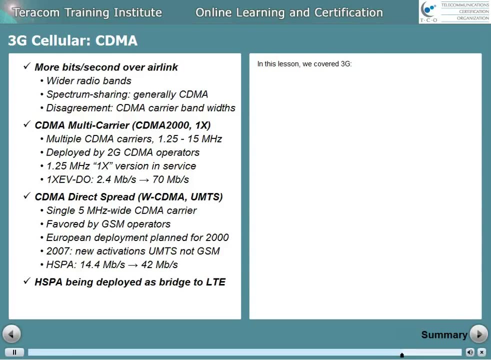 this was a major incentive for the 1X camp. It appears that one of the legacies of Steve Jobs will not just be the iPhone, but a key part in ending the cellular standards war. In this lesson we covered 3G. 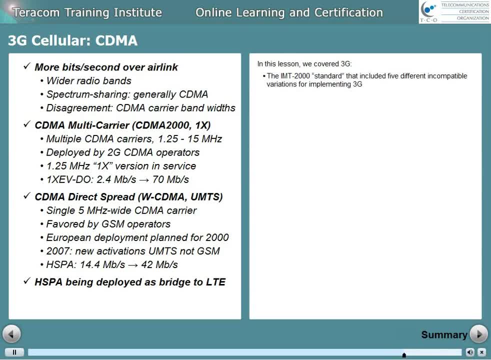 the third generation. We talked about the IMT2000 standard. that included five different, incompatible variations for implementing the third generation. The two that were of the most interest: IMT multi-carrier, also known as 1X, and IMT direct spread. 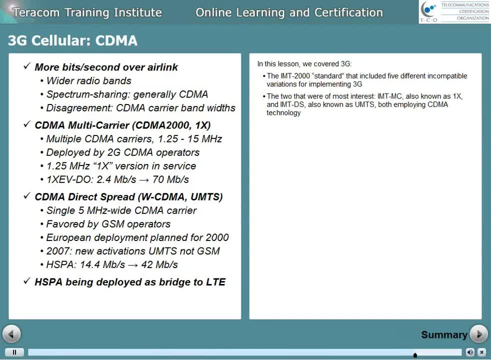 also known as UMTS, and both of them are CDMA technologies. We talked about the attempts to deploy UMTS without Qualcomm and without the United States GPS, which led to a seven-year delay in deploying UMTS. We covered the data-optimized versions. 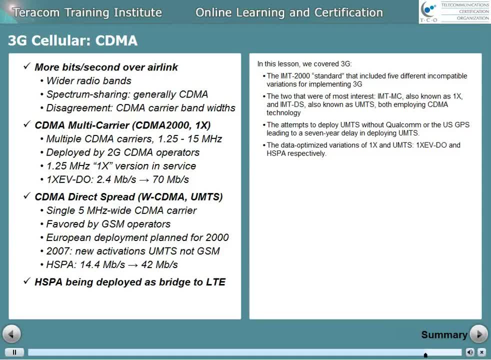 of 1X and UMTS. that's 1X, evolution, data optimized and high-speed packet access respectively. And we finished off talking about how market forces caused the capitulation of the 1X camp, deciding to go with the UMTS camp's. 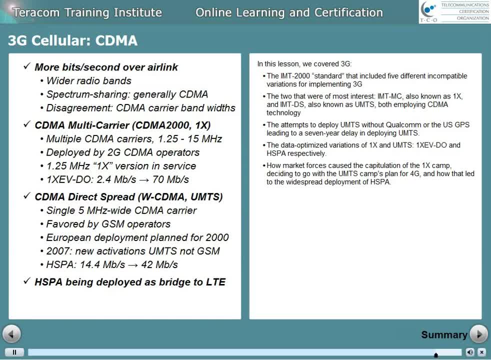 plan for 4G and how that led to the widespread deployment of HSPA, third generation data-optimized communications. Next are a couple of informal quiz questions to be sure you did not miss any key points, and then a quiz results screen. 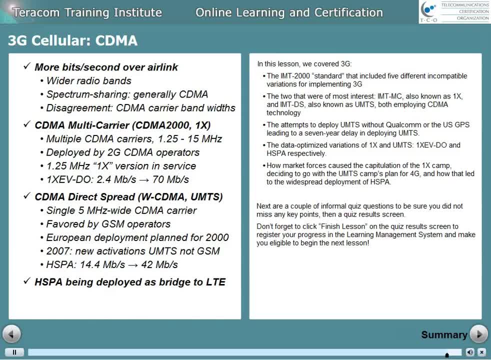 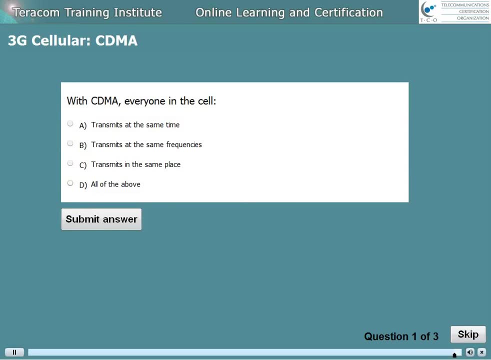 Don't forget to click finish lesson on the quiz results screen to register your progress in the learning management system and make you eligible to begin the next lesson. Thank you.